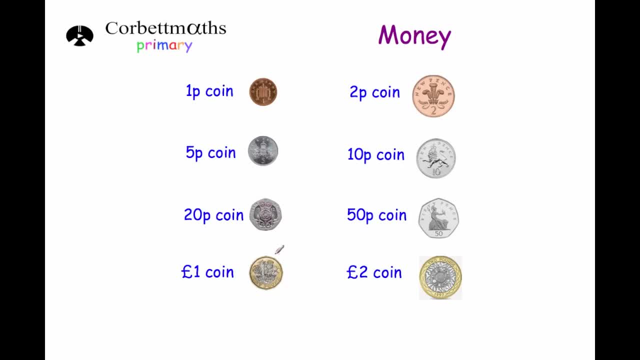 some special edition ones for those out. I haven't actually seen them yet, So I'm going to any yet, but they may come out in time- And the £2 coin. Okay, just one other thing that might be quite useful is to know how many of each coin we would need to make £1.. So with a penny we would. 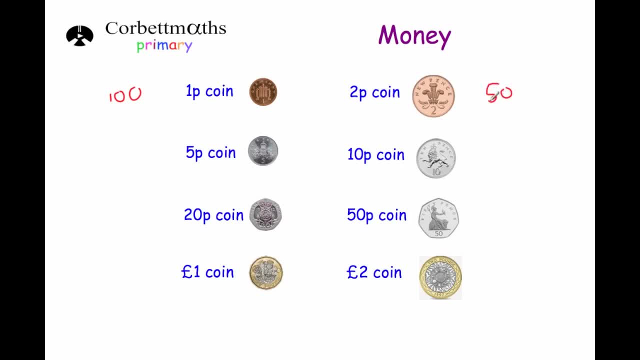 need 100 pennies to make a pound. We would need 50, 2p's to make a pound. We would need 20, 5p's to make a pound, 10, 10p's to make a pound, 5, 20p's to make a pound and 250p's to make a pound. 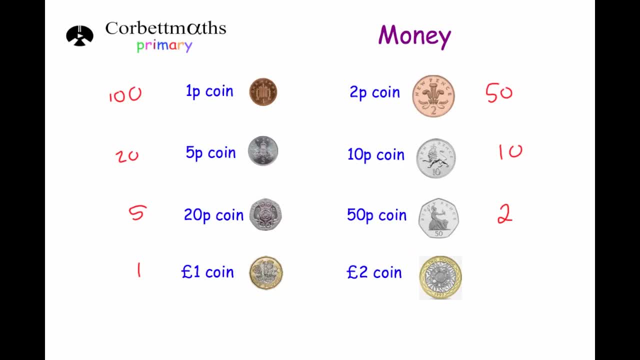 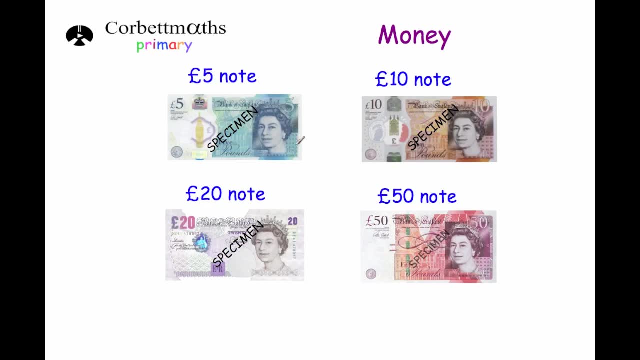 Obviously 1,, 1 pound and 2 pounds, obviously more than a pound Now. these are the current notes. at the moment We have got the £5 note, the £10 note, the £20 note and the £50 note. I believe in 2020 they're going to be bringing out the new plastic £20 note. 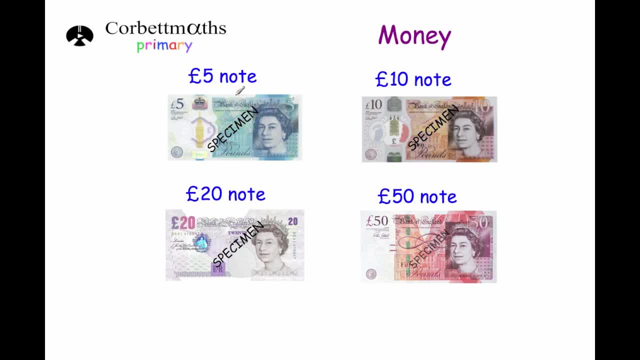 and I'm not sure about the £50 note yet, But as of 2018, these are the notes that are in current circulation, So the £5,, £10, £20 and £50 note. There are some other notes that are out there. 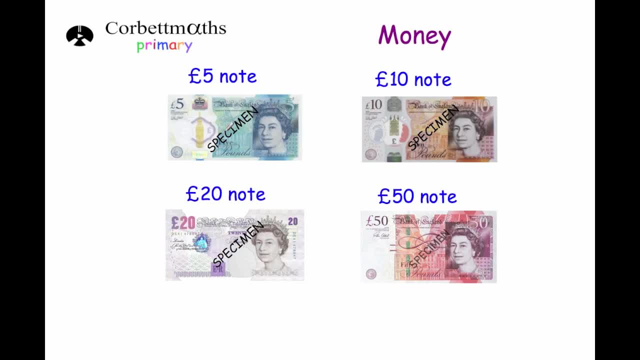 For instance, the Bank of Scotland's notes, Ulster Bank- sorry, Ulster Bank, for I'm trying to remember Northern Bank, Bank of Ireland. I should know the Northern Irish notes, But these are the main ones that are in the circulation within the. 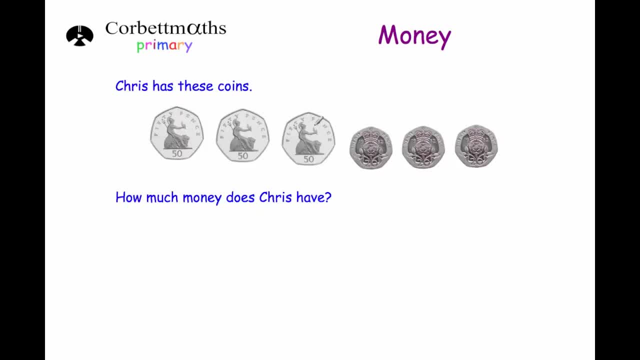 UK. Okay, let's have a look at some questions now. So here we have got a question. It says Chris has these coins. How much money does Chris have? So let's have a look at the coins. We have got 1,, 2, 3 50p coins and 1,, 2, 3 20p coins. So let's start by counting up the 50p coins We have. 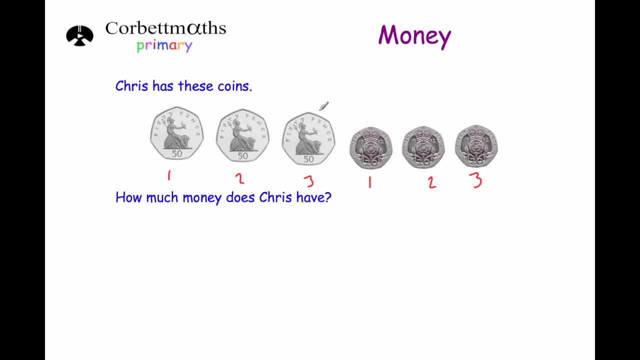 got £1, which is 50p, 2 of them which would be £1, and 3 of them which would be £1.50.. So we've got £1.50 in 50p coins, And then, in terms of 20p coins, we've got 20,, 40,, 60. So that's 60p, And then we 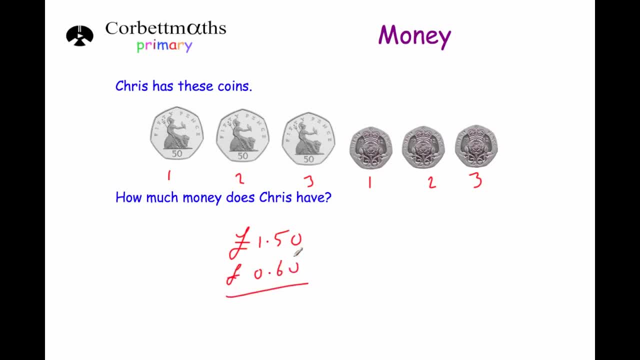 just need to add those together, The £1.50 in the 60p. So 0 plus 0 is 0.. 5 plus 6 is 11.. Put 1 down and carry the 1., And 1 plus 1 is 2.. So all together Chris has got £2.10p. 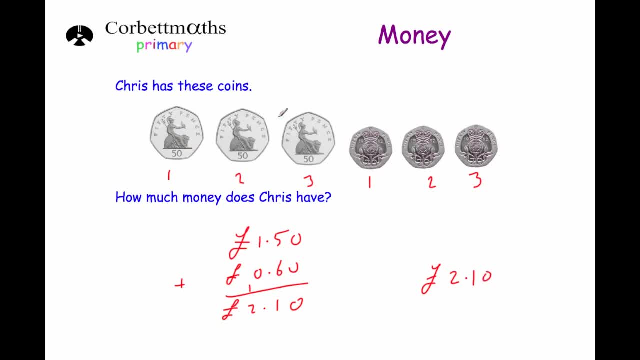 We could have just counted them up this way as well: 50p, £1,, £1.50,, £1.70,, £1.90,, £2.10p, by adding them up just as we go along. Okay, so that's quite a straightforward question. Let's. 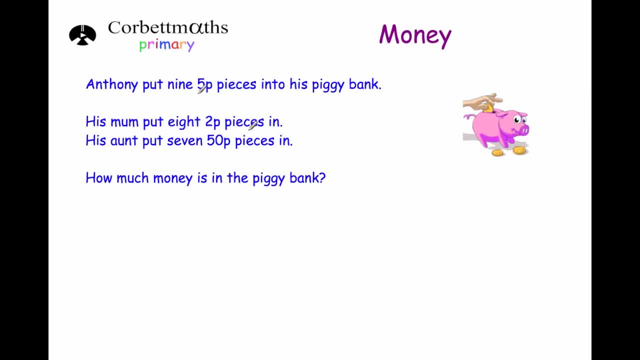 have a look at another one now, Right? so the next question says: Anthony puts 9 5p pieces into his piggy bank. His mum put 8 2p pieces in and his aunt put 7 50p pieces in. How much money is in? 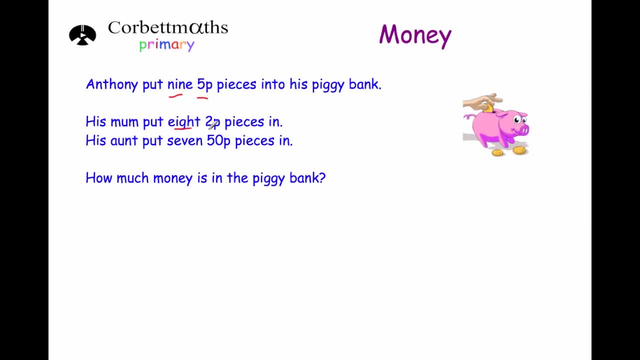 the piggy bank. So first of all we've got 9 5p's, 8 2p's and 7 50p's. So let's work out the total of each of those. So first of all with the 5p's. So 9 times 5p would be 9 times 5 is 45p. 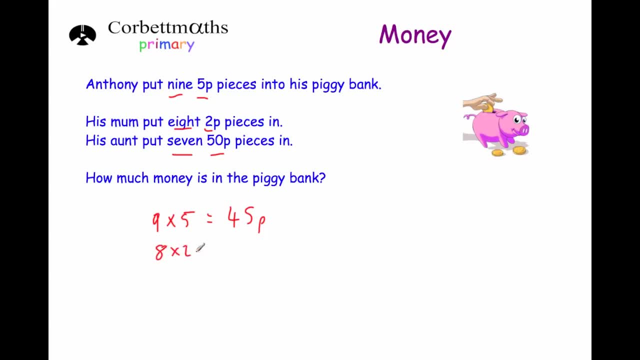 Next we have got 8 2p pieces. So 8 times 2 is equal to 16p. And then his aunt put in 7 50p pieces. So 7 times 5 is 35. So 7 times 50 would be 350p. That's the same as £3.50.. So let's add. 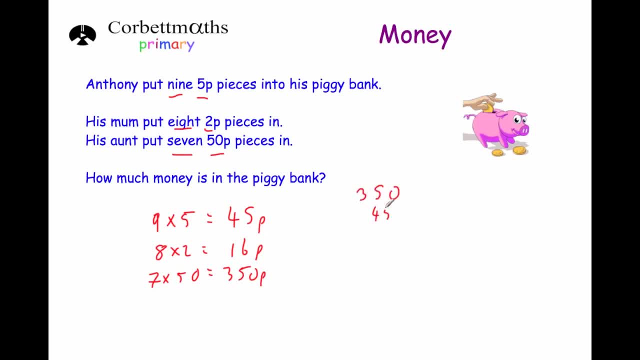 those together up first of all. So 350p, 45p and 7.5p, And if we add those up, 0 plus 5 is 5 plus 6 is 11. So put the 1 down and carry the 1. 5 plus. 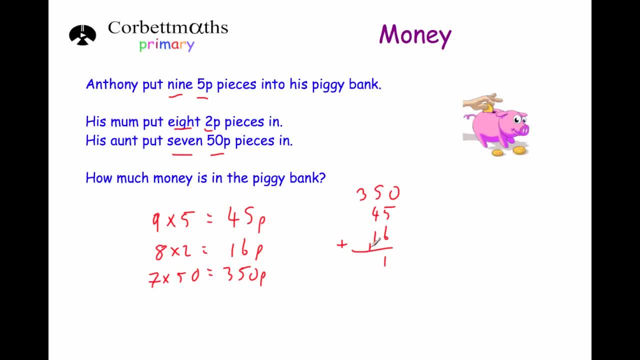 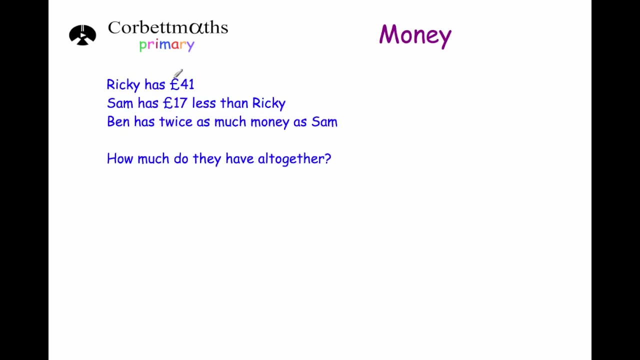 4 is 9 plus 1 is 10 plus 1 is 11.. So put the 1 down and carry the 1. And 3 plus 1 is 4.. So that's 411p or £4.11p, And that's it. Okay, let's have a look at our next question now. So this question. 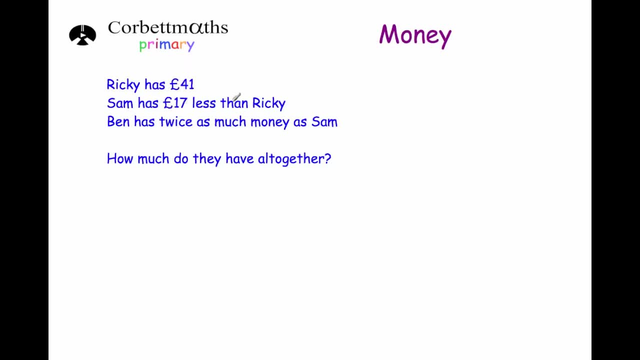 says: Ricky has £41. Sam has £17 less than Ricky And Ben has twice as much money as Sam. How much do they have all together? So first of all, we know that Ricky has Ricky. We've then got Sam and then we've got Ben. So Ricky has got £41. So he's got. 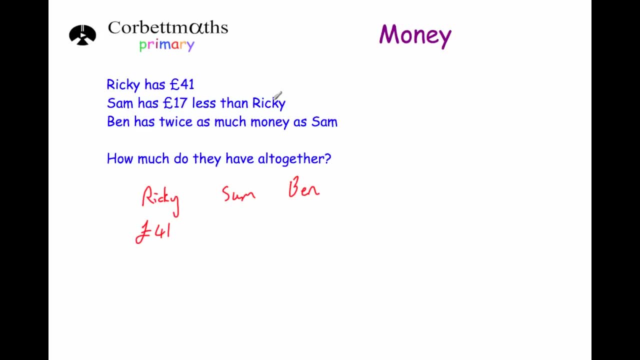 £41.. Sam has got £17 less than Ricky, So we're going to need to do £41 minus the £17 to see how much money Sam would have. So we're going to have to borrow one. So 11, take away 7 is 4.. 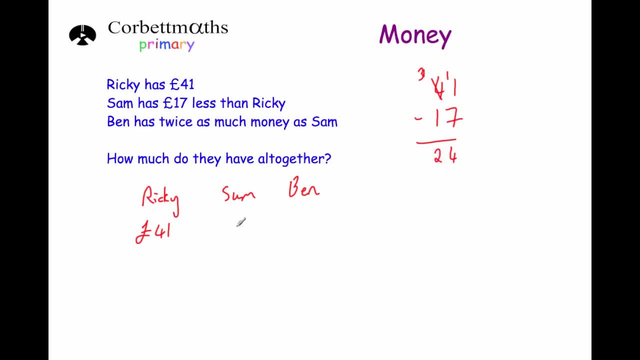 And 3, take away 1 is 2.. So Sam has got £24.. And it says Ben has got twice as much money as Sam. So if Sam's got £24, Ben will have double that. Okay, so we've got 24 multiplied by 2, which would: 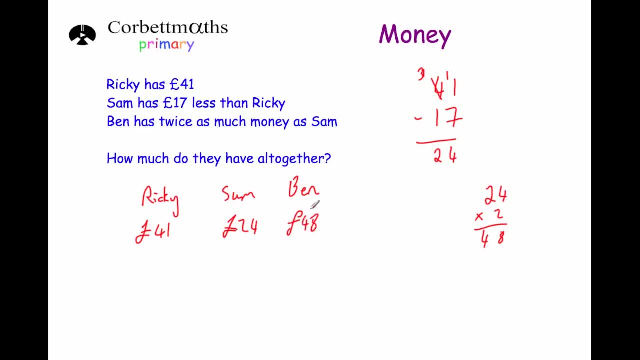 be £48. So Ben has got £48. So it says how much money do they have all together? So we just need to add together 48, 41 and 24.. And if we add those together we'll see how much money they have all. 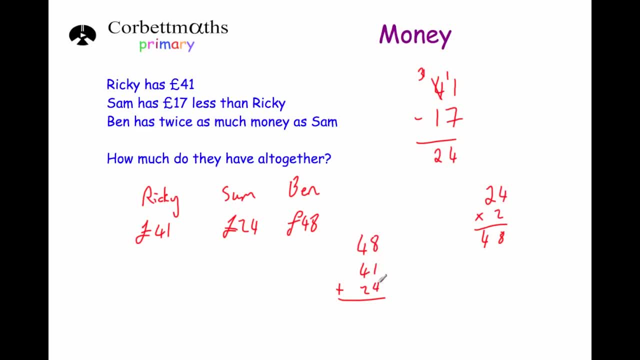 together. So 8 plus 1 is 4.. So we've got £48.. So we've got £48.. So we've got £48.. So we've got £49 plus 1 is 9 plus 4 is 13.. So put the 3 down, carry the 1.. 4 plus 4 is 8 plus 2 is 10 plus 1 is. 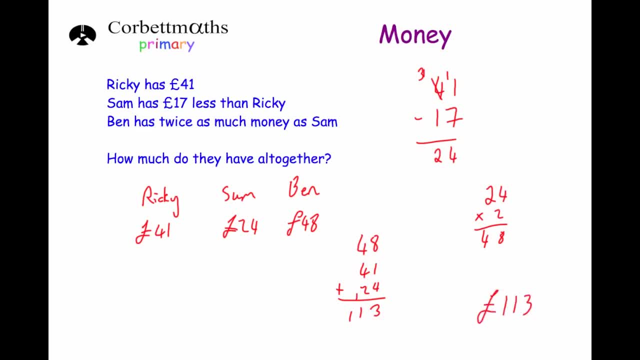 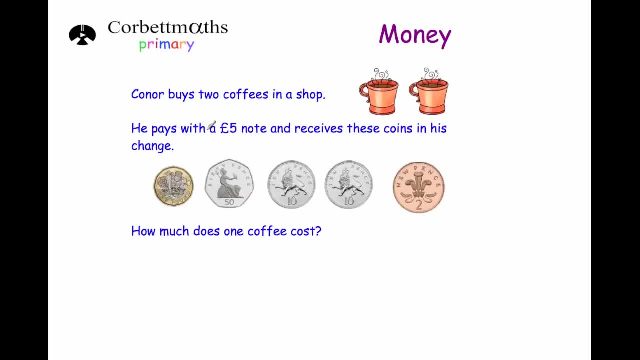 11.. So all together they would have £113.. Okay, our next question. So our next question says: Connor buys two coffees in a shop, He pays with a £5 note and receives these coins in his change. So this is his change And it says: how much does one coffee cost? So first of all, I'm going to 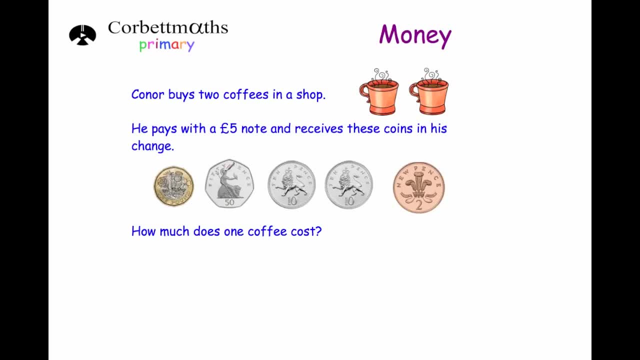 work out how much change he's received in total. So he's got £1.. £1.50, £1.60, £1.70, £1.72.. So he's received £1.72 change. So to find out how much money he's. 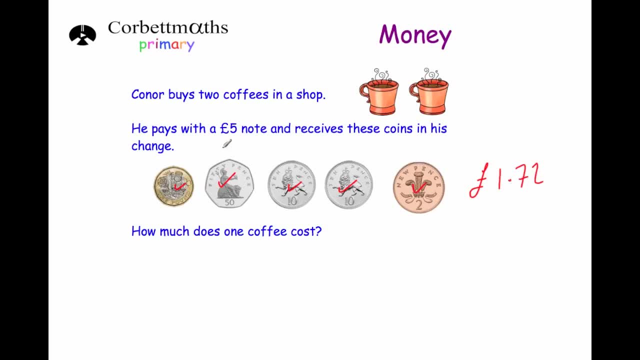 spent. we're going to need to take this £1.72 away from the £5 note, So £5 subtract £1.72.. And if we do that we'll see how much money he spent on coffee, And then we'll half that to. 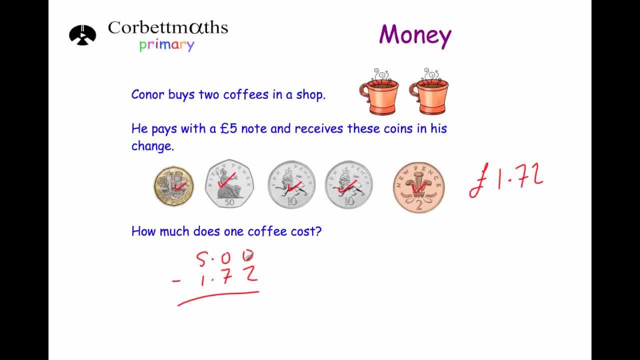 find the cost of one coffee. So to do that we're going to need to borrow, because obviously zero take away two we can't do. So we're going to borrow from the £5, call it a four and carry one over. We're then going to cross out the £10, call it a nine and put one there. So £10 take away two is 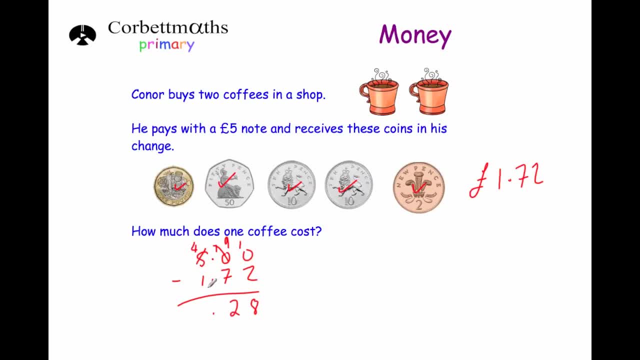 eight. £9 take away seven is two And £4 take away one is three. So all together Connor spent £3.28 on coffee. Now that's for two coffees, So to find the price of one coffee we're going to. 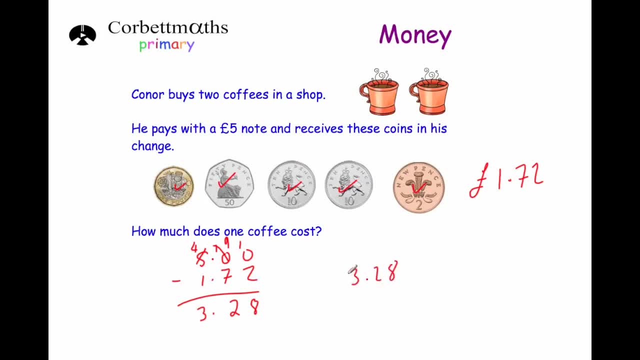 need to divide this by two. So we've got our £3.28 and we will divide that by two. So two into three goes once remainder. one, Two into 12 goes six times and two into eight goes four times, So each. 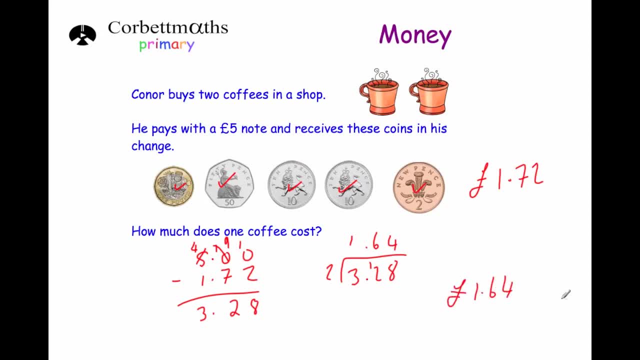 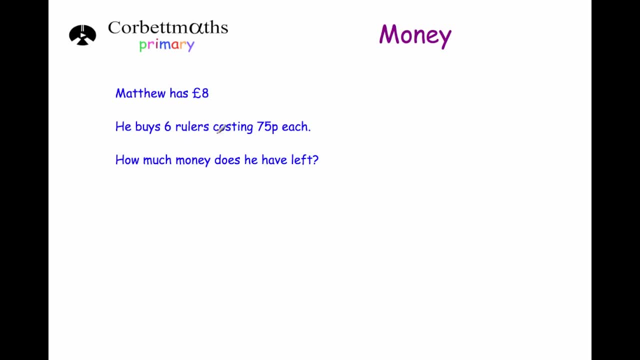 coffee costs £1.64 and that's it, Okay. our next question. Our next question says: Matthew has £8.. He buys six rulers costing 75p each. How much money does he have left? Okay, so we're going to need to find out how much money Matthew spent on rulers in total. So the six rulers costing 75p each. 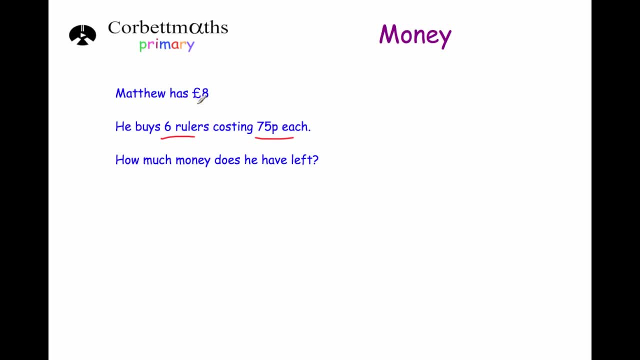 So we're going to divide these together. We'll see how much money he spent on rulers and then we'll take that away from the £8.. So we're going to do 75 multiplied by six. So six times five is 30.. Put the: 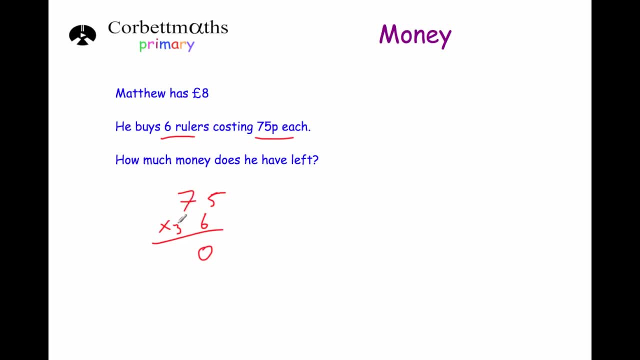 zero down. carry the three Six times seven is 42 plus three is 45. So all together, Matthew spent £450, which is £4.50.. So now we need to take that away from the £8.. So we're going to do £8. 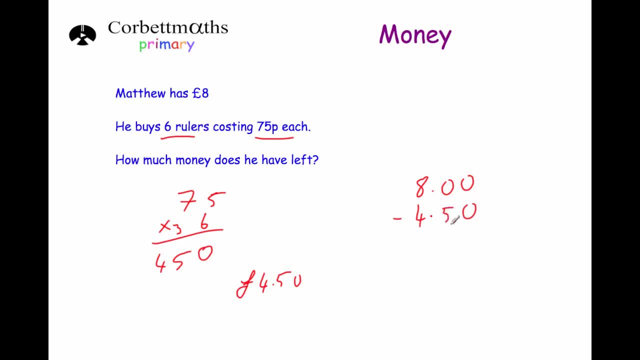 subtract £4.50 to see how much change he was making. So we're going to do £8 subtract £4.50 to see how much change he was making. So we're going to do £8 subtract £4.50 to see how much change he was making. So we're 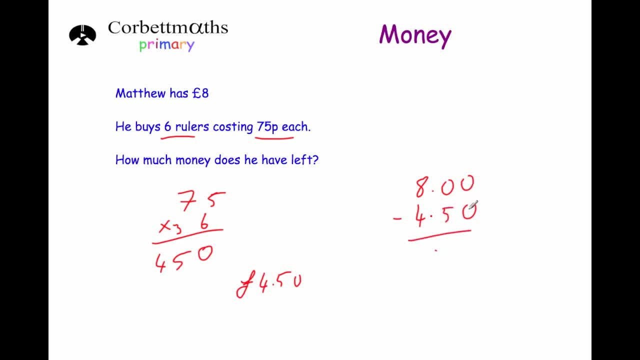 get or how much money he had left. so zero take away zero is zero. zero take away five. we're going to need to borrow one, so call that seven and ten. so ten take away five is five, and seven take away four is three. so all together, Matthew would have three pound fifty left right. our next question. 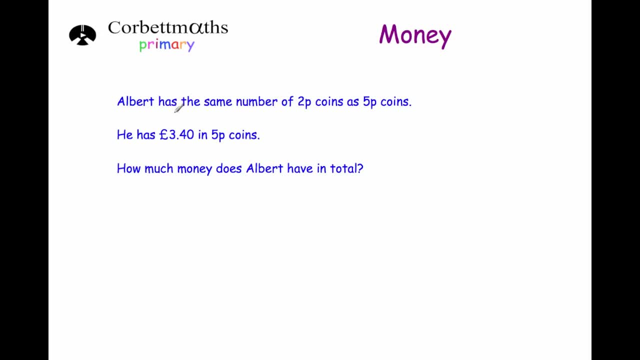 this is our second last question. Albert has the same number of two p coins as five p coins, so he's got the same number of coins. he has three pound forty in five p coins and the question says: how much money does Albert have in total? so what we're going to do is we're going to find out how. 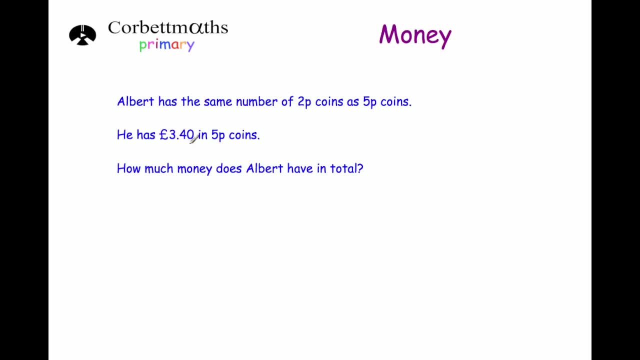 many five p coins Albert has has us in total to begin with. okay, so we've got three pound forty. if we divide that by five we will see how many five p coins he's got. so we're going to write 340 pence and we're going to divide that by five pence. so five into three doesn't go remainder. 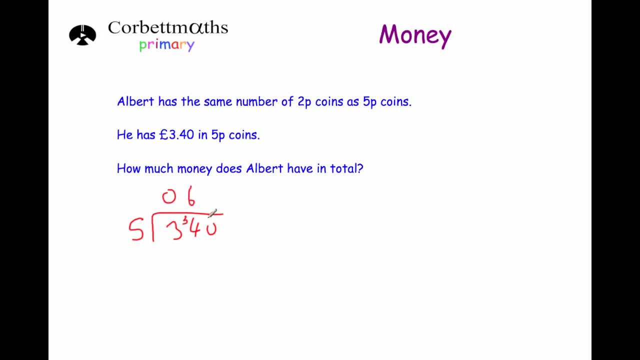 three. five into three doesn't go. remainder three, thirty four goes six times through my remainder four and five into forty goes eight times. so altogether he has sixty eight five p coins. okay, so it says he is the same number of two p coins as five p coins. that means he will have sixty eight five p coins, so that, and that means he'll. 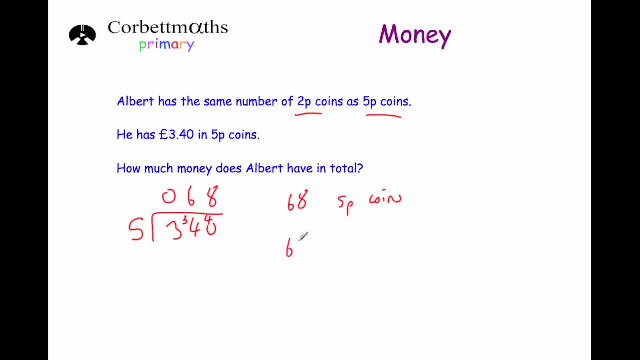 also have sixty eight, two p coins. so we're going to do sixty eight times by two to see how much money he has in two p coins. so let's work that out. so sixty, sixty eight multiplied by two, so eight times two is sixteen. put the six down, carry the one. 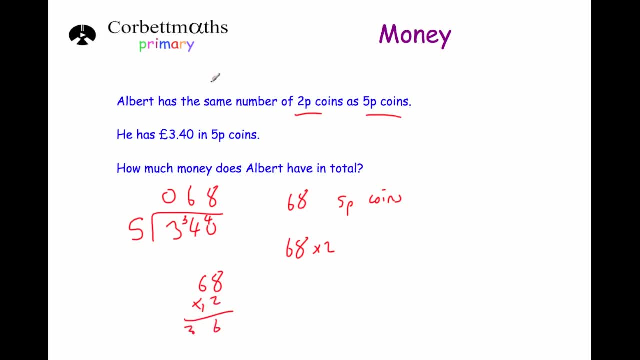 two times six is twelve plus one is thirteen, so he altogether he would have one pound thirty six in two p coins. that says how much money does he have in total. so we've got the three pound forty in the five p coins and we have got also here albert's also got the one pound thirty six in. 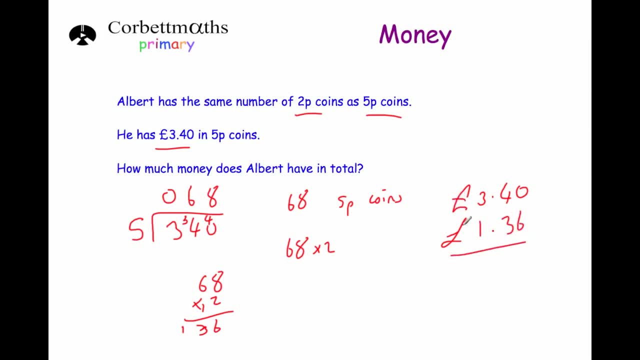 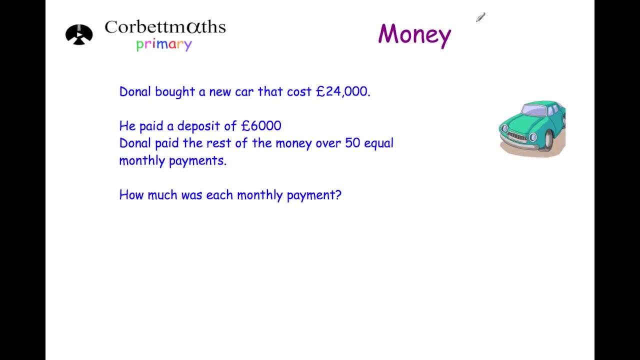 two p coins and if we add those up together, we've got those together. we'll see how much money he has in total. so zero plus six is six, four plus three is seven, and three plus one is four. so altogether albert would have four pound seventy six, right? so our last question? so our last question says donald. 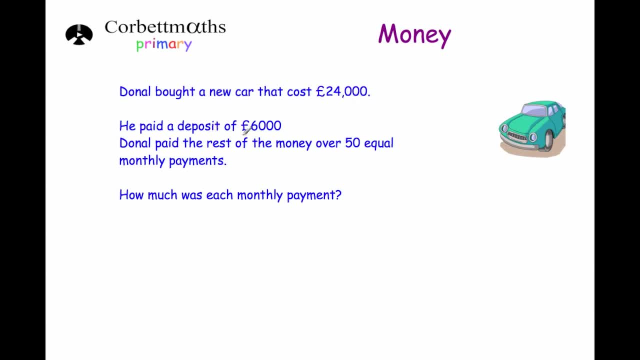 bought a car that cost twenty four thousand pound. he paid a deposit of six thousand pound and donald paid the rest of the money over fifty equal monthly payments. how much was each monthly payment? so the car cost twenty four thousand pounds and he paid a deposit of six thousand pounds. so if we're 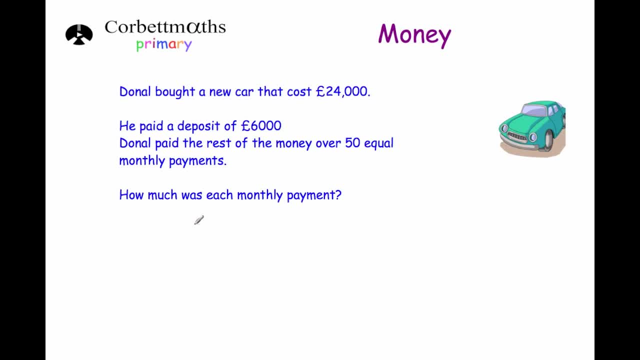 take those away. we're going to see what's left to pay. so twenty four thousand pound, take away six thousand pound. well, if we do that, we're going to get uh, four, take away six. we can't do so, we're going to borrow. we're going to get eighteen thousand pound. so this eighteen thousand pound. 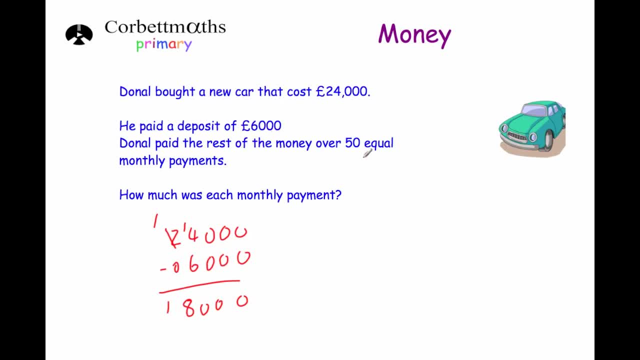 left to pay after his six uh thousand pound deposit. and he pays that fifteen uh, that eighteen thousand pound over fifty equal monthly payments. so if we divide eighteen thousand by fifty we'll get the amount of each monthly payment. so eighteen thousand divided by fifty, fifty into one doesn't go remainder one. fifty into eighteen doesn't go remainder eighteen, fifty into. 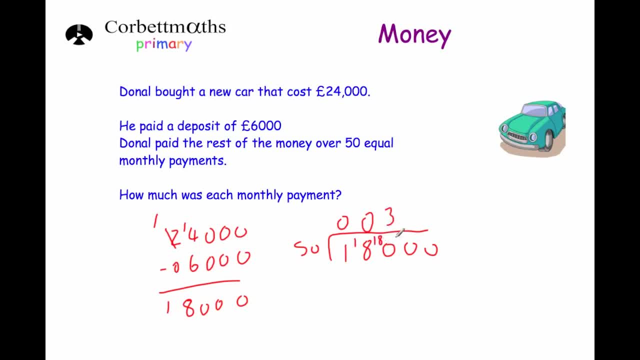 one hundred and eighty goes three times, remainder thirty, because three fifties are one hundred and fifty and with one hundred and eighty there'll be a remainder of thirty. fifty into three hundred goes six times and fifty into zero goes zero times. so how much was each monthly payment, each monthly? 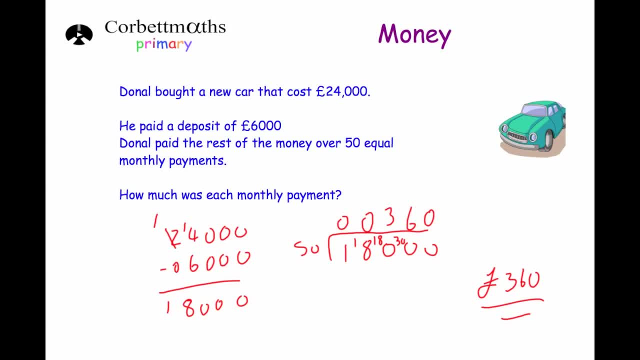 have been three hundred and sixty pound, and that's it.